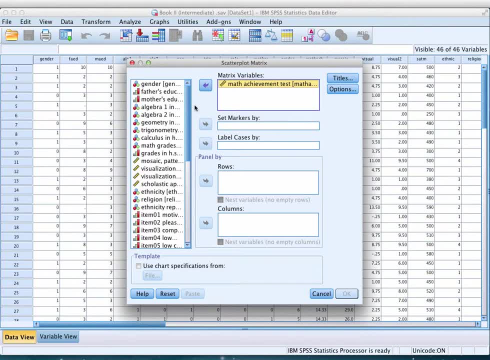 variable. we want to see the relationship with it and the other predictor variables. We can add an operator up here and we're going to use that to look for a variable and we'll do that in our model that we're going to use. So we have a figure we're going to use here and then we'll look at the test and we're going to 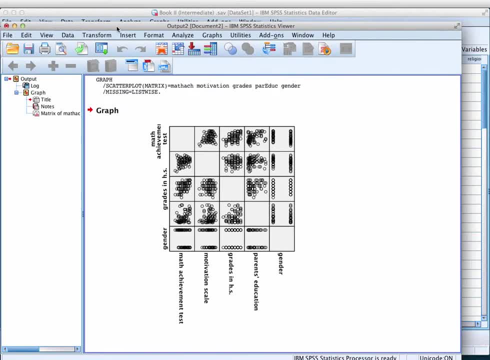 check for the model we want to use- and again, we'll talk about that in just a moment. So we're going to click on, we're going to check the error, so we're going to go to the math constellation and we're going to go to the finals and we're going to be able to find the variable that we want. So, again, if you're going to be, 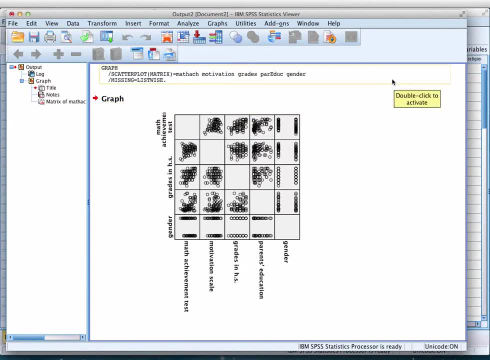 relationship or the pattern of relationship between our dependent variable, math achievement, in our predictor variables or independent variables. and you can see, with the motivation scale we could superimpose a line within this massive data points. same way, with grades in high school, we could superimpose a line here for parents, education, we can superimpose a 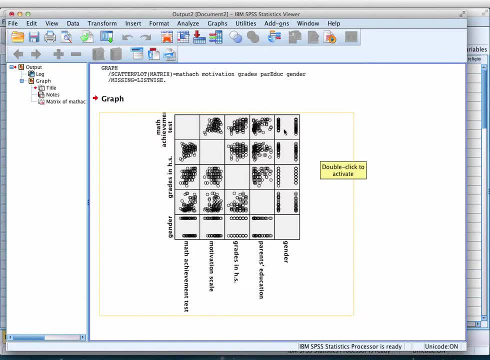 line here, although this is somewhat curvilinear, and, of course, for gender there's no line that we can really superimpose, because this is categorical data and so, as you recall, this data is score is coded as 0 for female and one for males. so that gives us an idea about our assumption of linearity between the 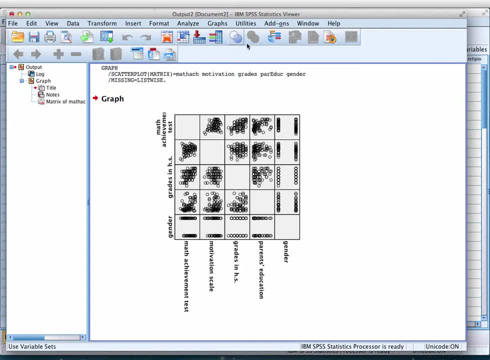 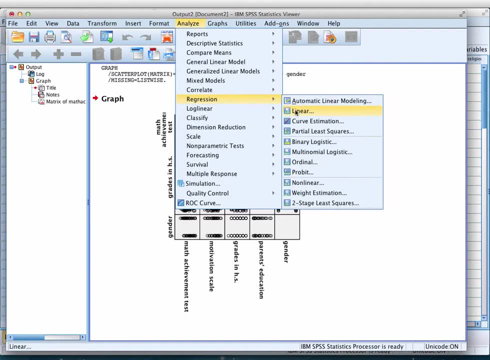 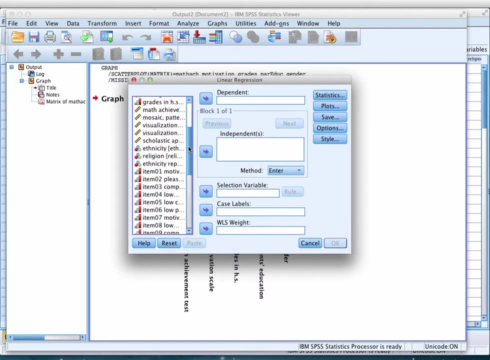 dependent variable and the independent variables. now we can go up and run our regression analysis. so we go to analyze regression and then linear and in this case for dependent variable. we want to have a math achievement in this box and then we're going to put in motivation grades in high school parents. 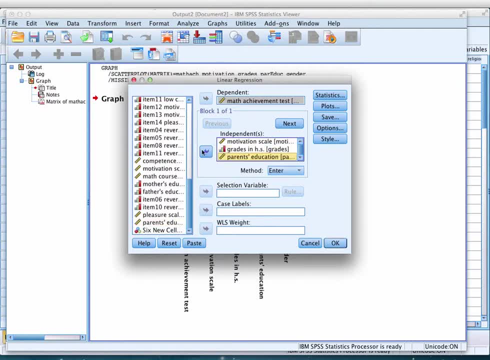 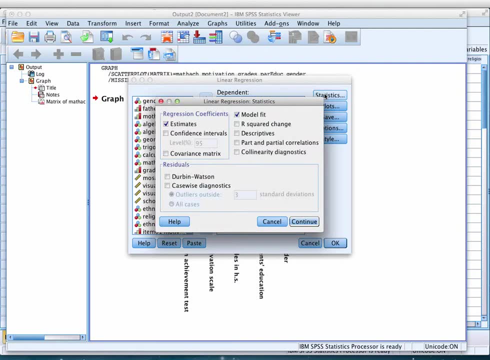 education and gender. now for statistics. we want to make sure that estimates and model fit is checked now the. this is checked by default in SPSS, and one other thing we can do is check descriptives, because that will provide us with the correlation coefficients or the correlation matrix. 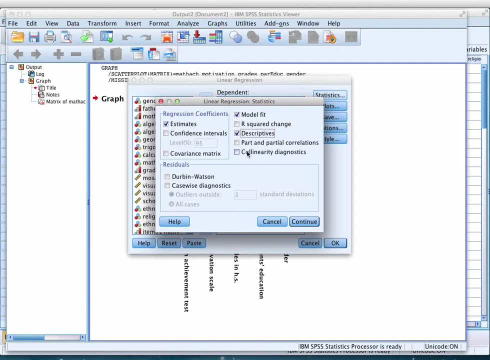 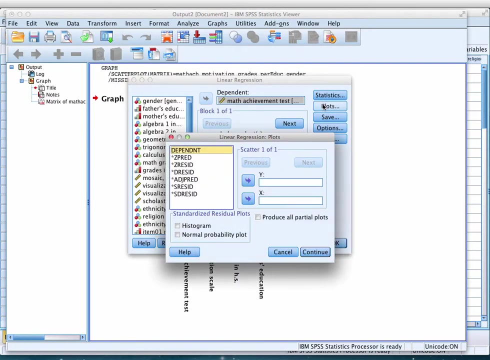 between the dependent and independent variables, and then the collinearity diagnostics, because another assumption of multiple regression is that we don't have the issue of what's called multi collinearity, or when variables are highly correlated with one another in terms of plots. diagnostically, we like to look at the relationship between the predicted 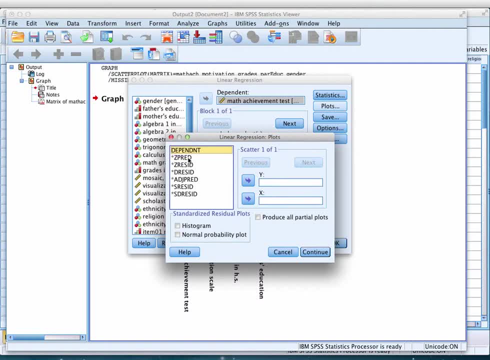 values and the residuals, and so we want to move the Z of the predicted values to the Y box and the Z of the residual values to the X box. so these are standardized, and that makes it easier for us to look at these things graphically, and then we can click on histogram because we want to. 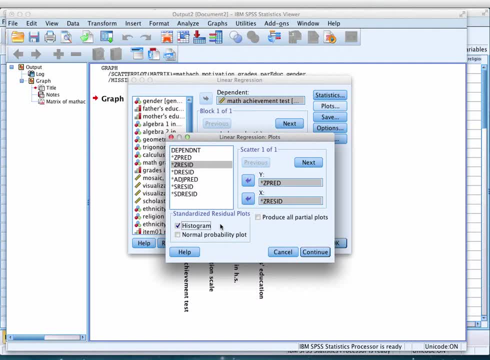 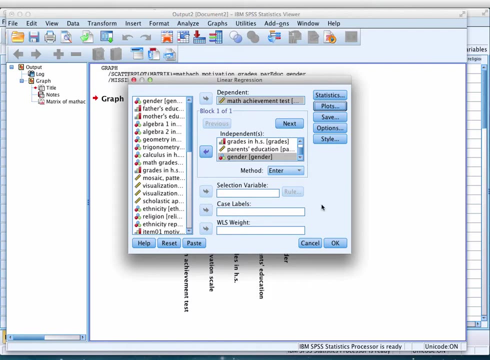 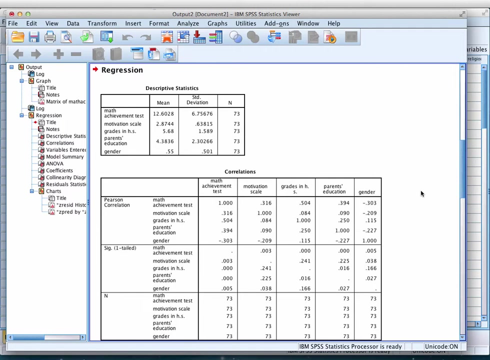 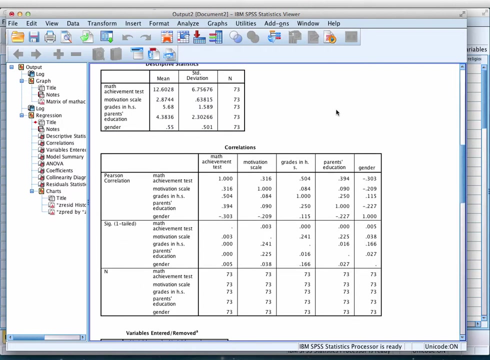 see if our residuals or if the error is normally distributed. that's also one of the assumptions that ANOVA- I'm sorry, multiple regression- follows continue and then we can run our analysis. so you see, by checking descriptives we get the means and the standard deviations for the variables that were analyzing and then 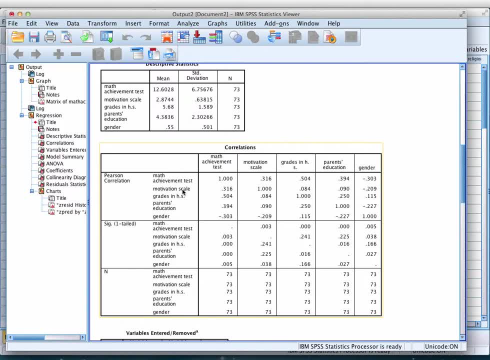 for the correlation matrix. we get the Pearson correlations and it's interesting to look at how each of our dependent variables are. each of our independent variables correlates with our dependent variable. So these correlate fairly well. They're not too high and they're not too low. And then you can see how the other independent variables correlate with. 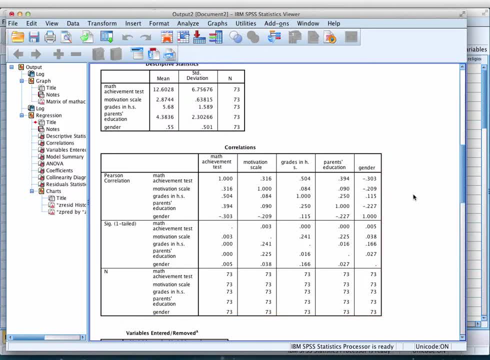 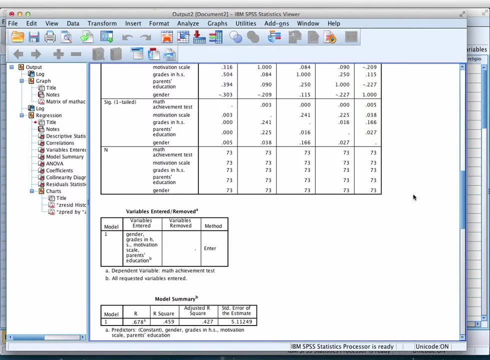 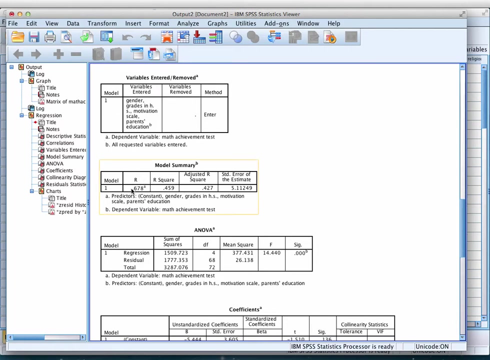 one another And we don't want independent variables to be highly correlated, Otherwise they're duplicating or they're overlapping. They're not providing unique variance to explaining, in this case, math achievement. When we look at the model summary, our coefficient of determination was point six, seven, eight or almost point six, eight, and our square is point. 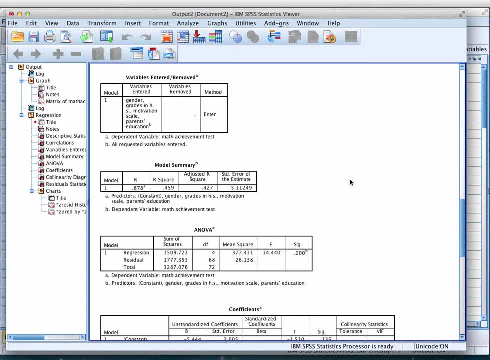 four, five, nine. So what this means is that forty-five percent of the variance in math achievement is explained by the linear equation. So we're going to use the linear equation to calculate the linear combination of gender grades in high school motivation and parents education. 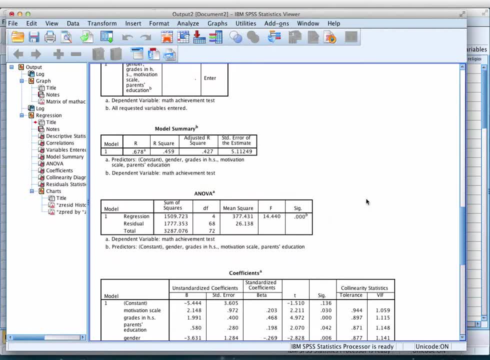 We also see that the ANOVA summary table is providing us with our regression sum of squares. So this is the variability that's explained, The error or residual that's not explained. And so four divided into 15 minus 15 is equal to one. So we're going to use the regression sum of squares. 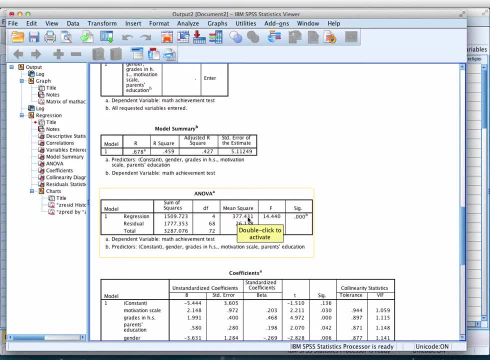 So this is the variability, that's explained, The error or residual, that's not explained. So the error or the regression sum of squares One plus five plus one zero nine is three, seven, seven point three, one Sixty-eight divided into one, seven, seven point three, five, eight is twenty six point one three, eight. 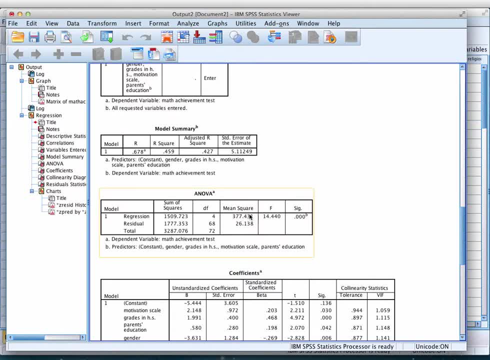 So the ratio of the regression, the explained variability, to the unexplained variability, is fourteen point four. So this is a large F ratio, and what it means is that that linear combination of variables is explaining a math achievement beyond chance levels. So this is not just by error, but this is 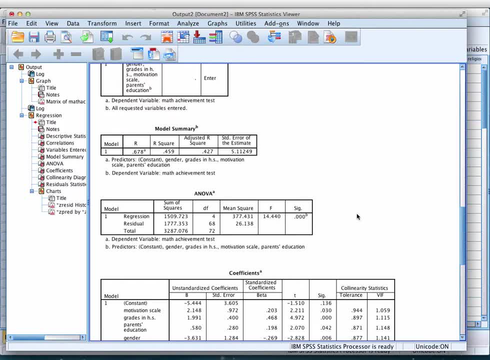 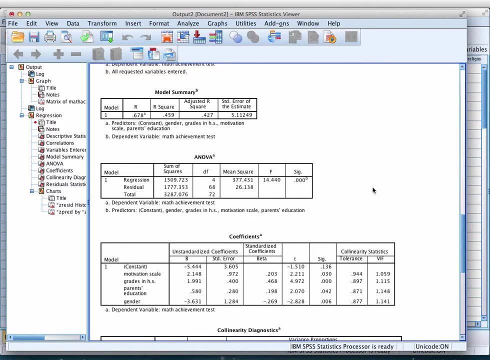 a rigorous and a robust explanation of these by these independent variables. So now what we need to do is figure out which variables provide the most contribution to explaining math achievement. So we can see here in the coefficients table we have our what are called unstandardized coefficients. So 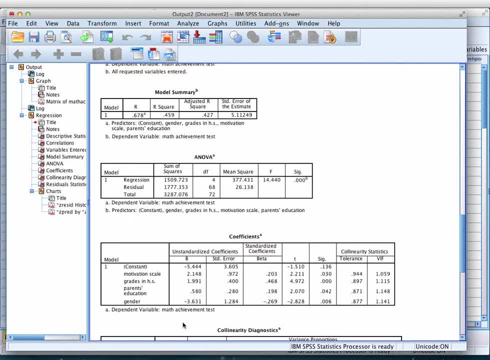 these variable. these coefficients are based on the scale, or the measurement scale for each one of these separate variables. The standardized coefficients, however, are based on a mean of zero and a standard deviation of 1.. So what that means is that we can compare these coefficients to determine which ones have the largest influence or 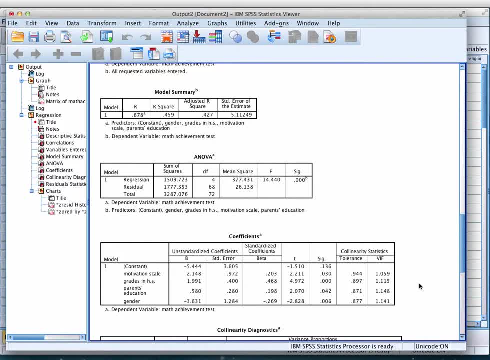 effect on math achievement. So if we look, we can see all of these contribute significantly to explaining math achievement. And here that, even though they're all significant, this tells us this one is the most important because it's the largest coefficient, followed by, followed by gender. so we don't look at this as being high or low. we we interpret the absolute. 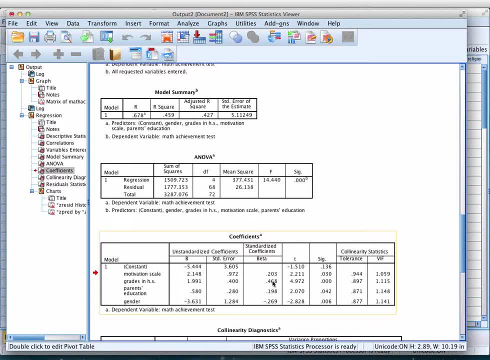 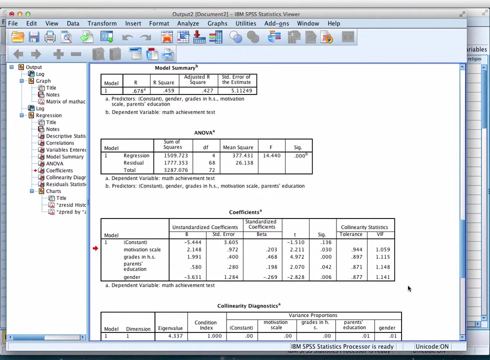 value. so grades in high school is the most important, followed by gender and motivation, and then parents education. the tolerance tells us a little bit about multi-coloniality, and so what that means is how these independent variables relate to one another. so, for example, if we took gender and made that 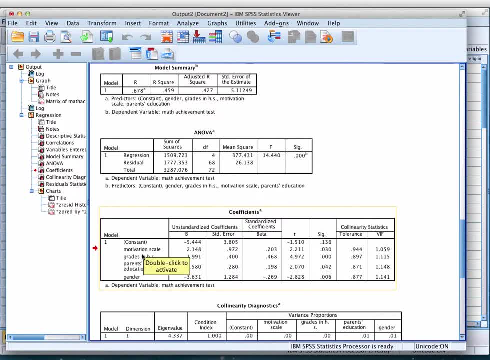 our dependent variable and let motivation grades in high school and parents education be independent variables. this would tell us how closely those variables are related to one another, and we can see that in this case our tolerance is 0.877. rule of thumb is tolerances that are closer to one could. 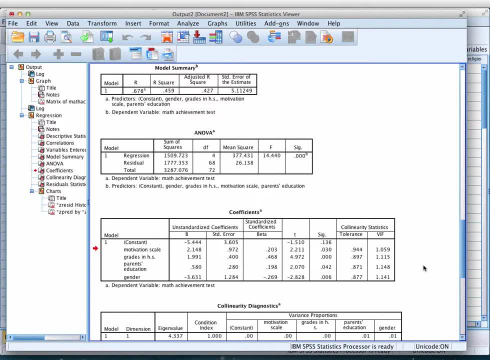 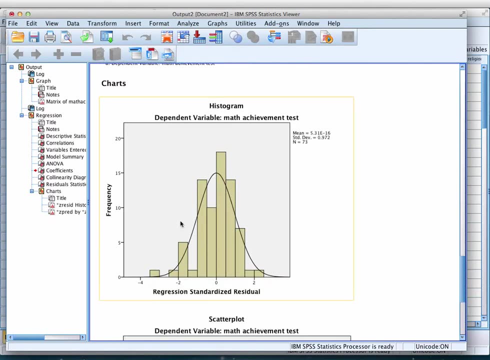 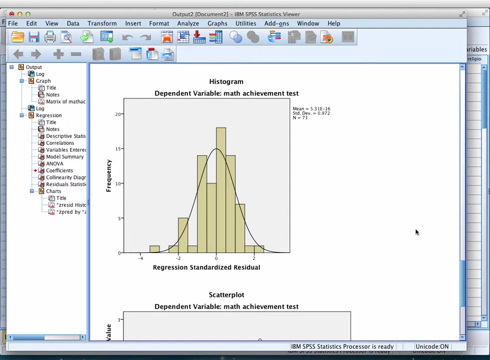 be problematic. tolerance is closer to- I'm sorry- tolerance is closer to zero can be problematic. tolerance is closer to zero can be problematic. tolerance is closer to one are better. this table, I'm sorry. this figure shows us the distribution of our residuals or error, and we can see that in this case the error is normally distributed so.